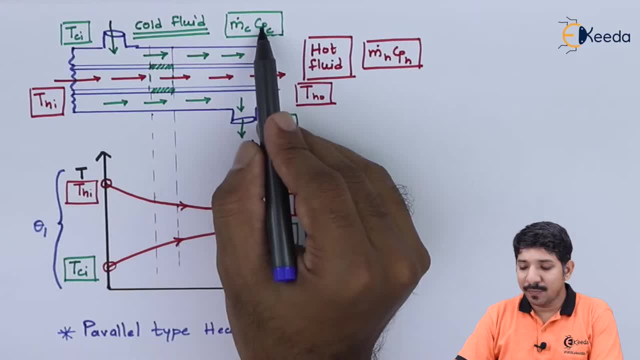 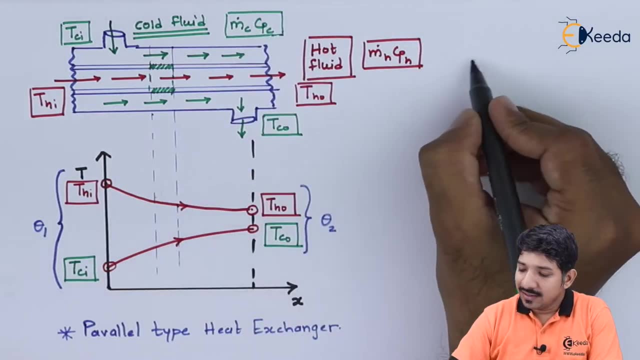 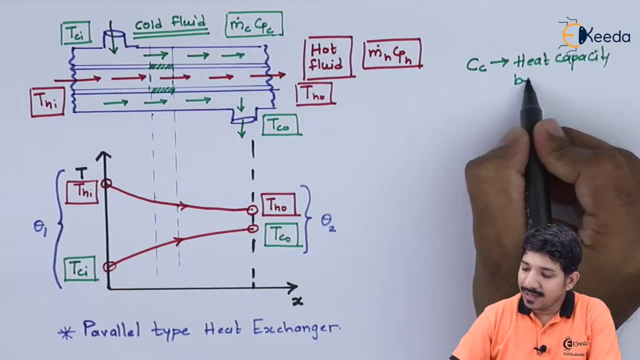 Similarly, the mass flow rate and the specific heat for the cold fluid is given as MC and CPC. So basically they call CC, that is the heat capacity by cold fluid, and this capital CC is nothing but MC and CPC. So this they have done simply for sake of the ease of analysis in case of a LMTD method. 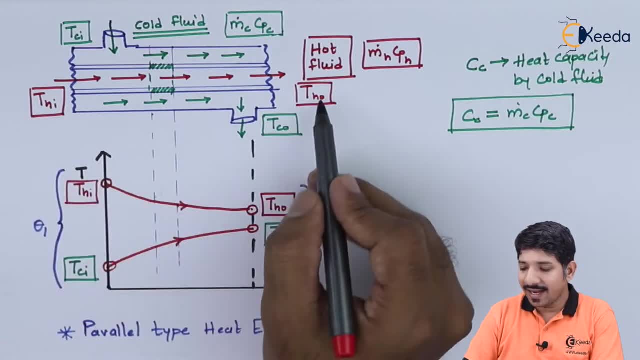 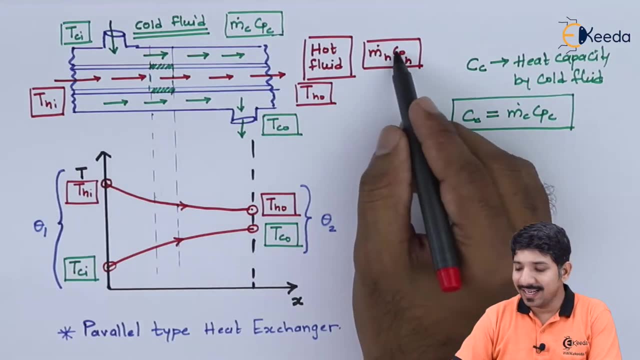 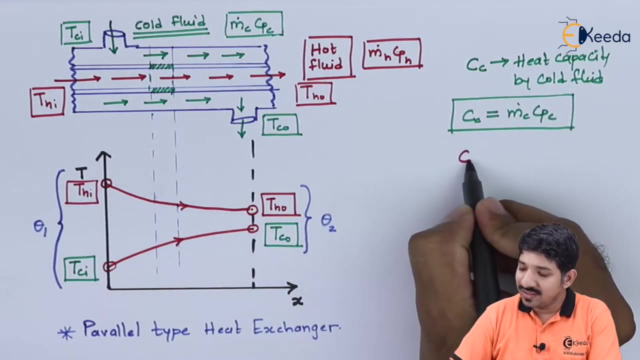 Similarly, the hot fluid inlet temperature is THI and the exit temperature is THO. The mass flow rate of the hot fluid is MH and CPH is the specific heat, Just like the CC, That is, the heat capacity of the cold fluid. 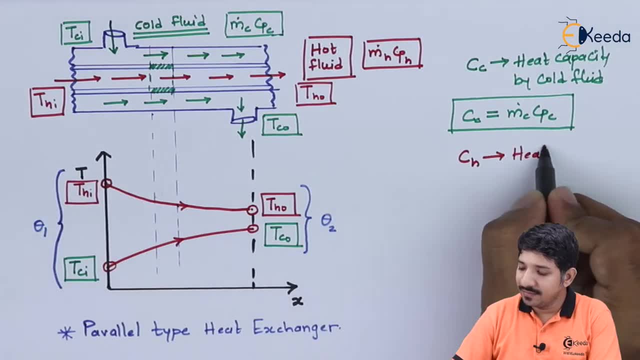 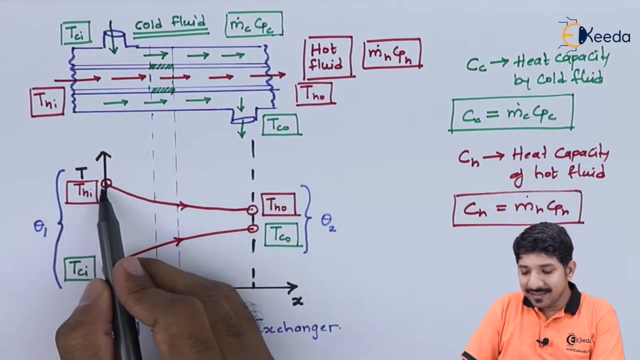 CH is nothing but the heat capacity of hot fluid. So we can write this: CH is nothing but MH and CPH. Now let us look at what is happening over here. This point indicates the inlet of the hot fluid, That is, THI. 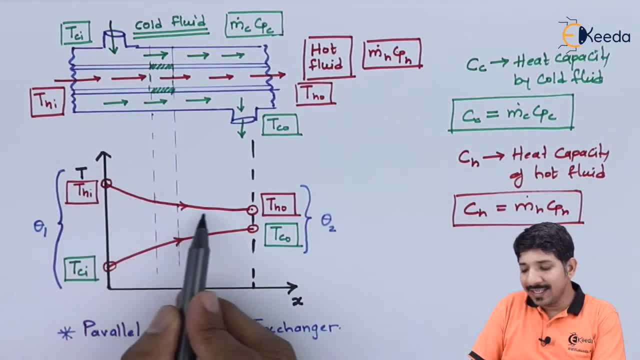 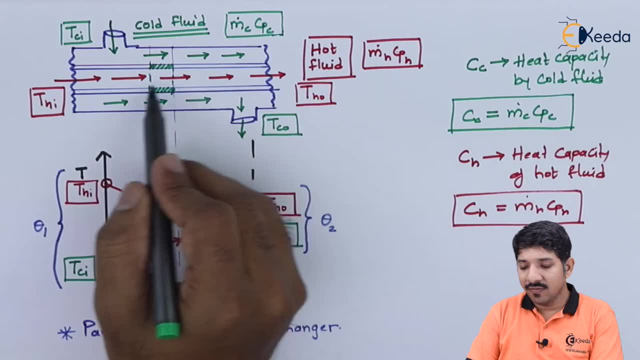 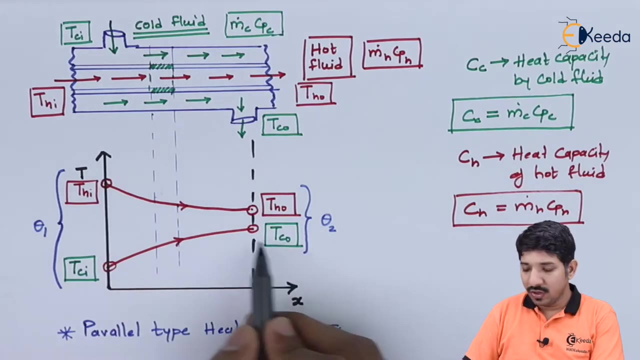 And then, parabolically, the temperature of the hot fluid will decrease till it reaches to THO. Similarly, since it is a parallel flow, so both the hot and cold fluid will follow the same direction: The cold fluid will enter at TCI and it will exit at TCO. 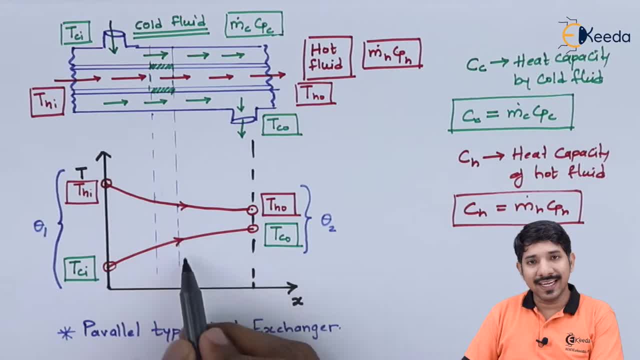 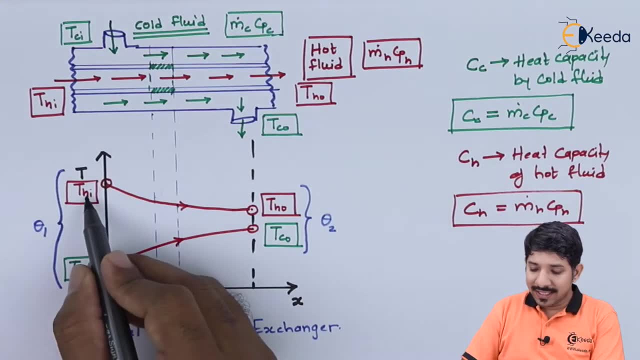 So we need to make sure that the arrows are put rightly on this diagram of T versus X for the parallel flow heat exchanger. Now, THI minus TCI indicates THETA1.. Now again, this is done for the sake of simplification. 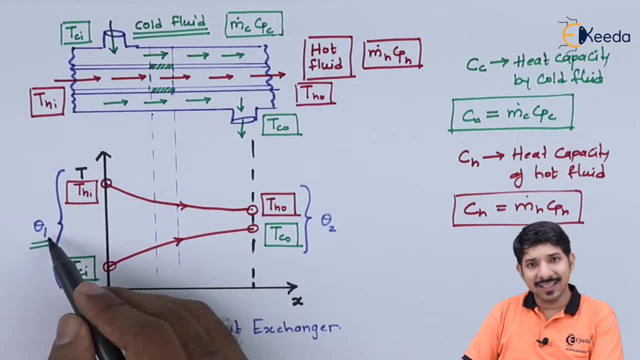 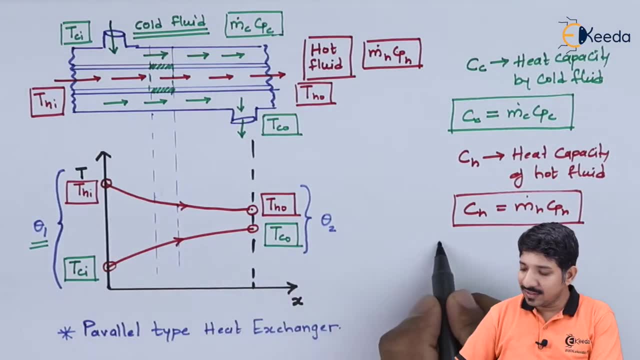 So the difference between the inlet temperature of hot and cold fluid is given as THETA1 and the difference between the exit temperature of hot and cold fluid is given as THETA2.. So obviously we can write it down here: THETA1 is THI minus TCI and THETA2 is THO minus TCO. 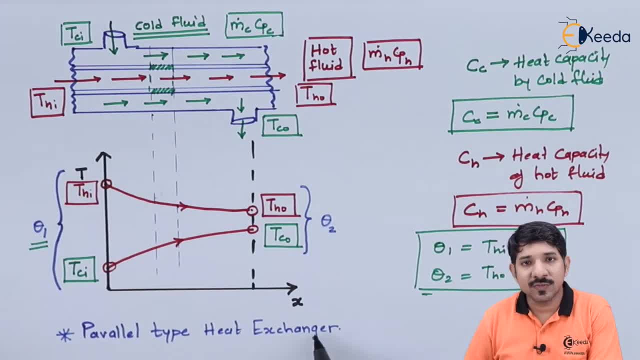 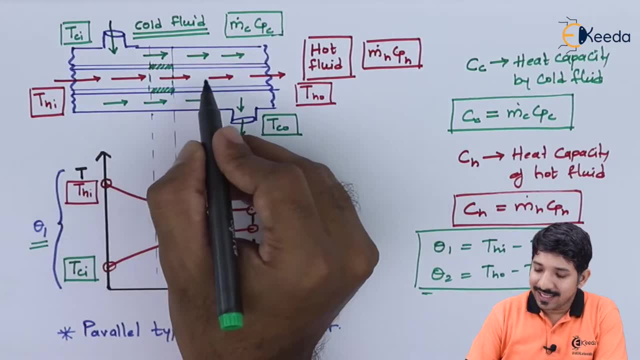 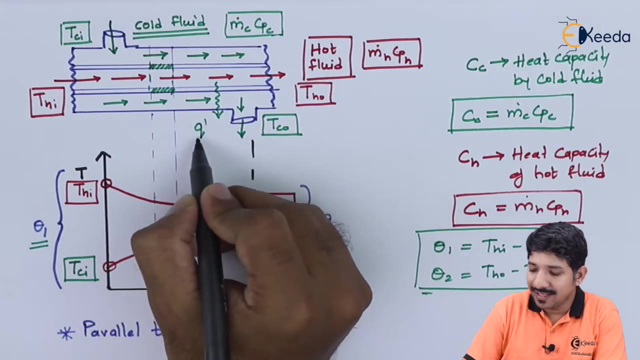 Now let us start the derivation of the same. If I assume that the heat transfer rate in this case, that is, from the hot fluid to the cold fluid, is given, as, let's say, this heat transfer rate is Q, dash, then how to find? 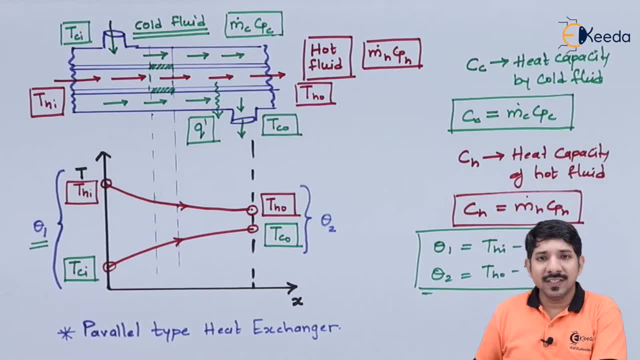 this heat transfer rate. There are three ways by which we can find the heat transfer rate here. One is using the overall heat transfer coefficient, and then the other two ways are nothing but the enthalpy difference between the hot fluid and the enthalpy difference between the cold. 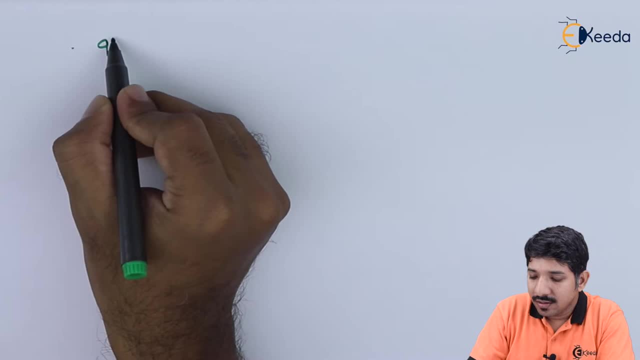 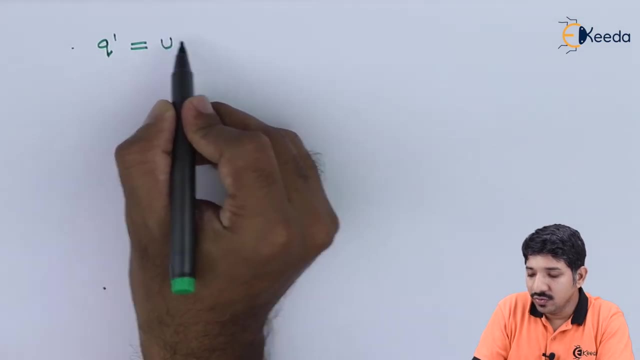 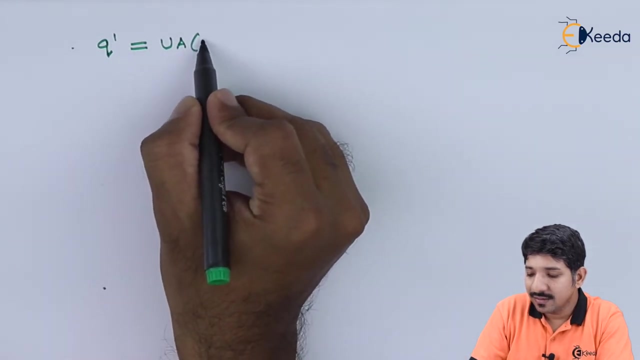 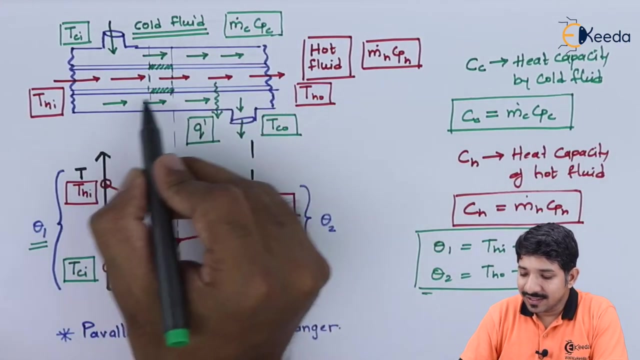 fluid. So let us write down the value of Q dash, that is, the heat transfer rate in case of a heat exchanger, is given as UA and the temperature difference is, let's say, TH minus TC. Now here what we have done: We have considered the 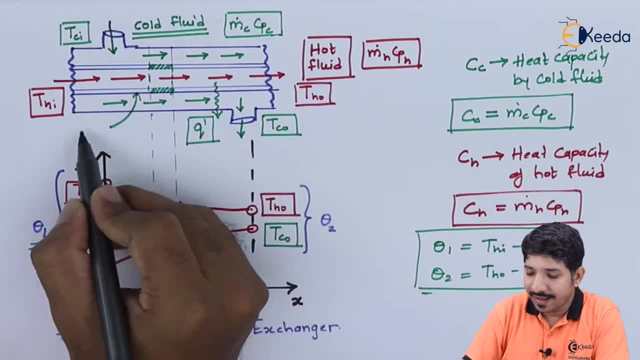 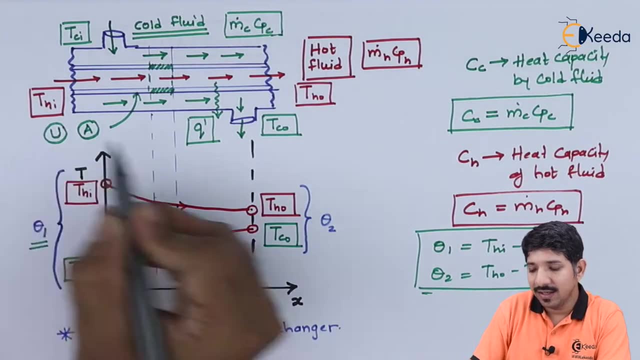 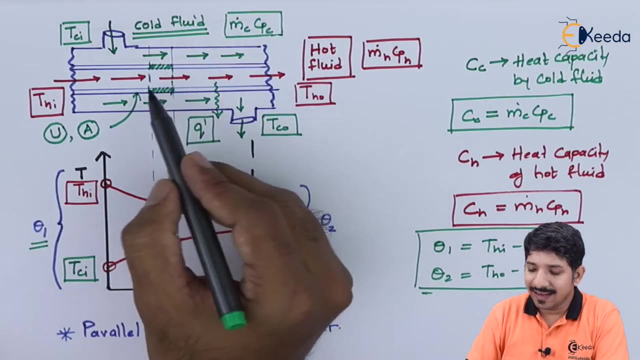 Area as A. now this is my surface area- and the overall heat transfer coefficient in this case is, let's say, capital U. So this is my assumption for the given metal. Similarly, we have assumed that for instantaneous, the hot temperature is given as TH and the 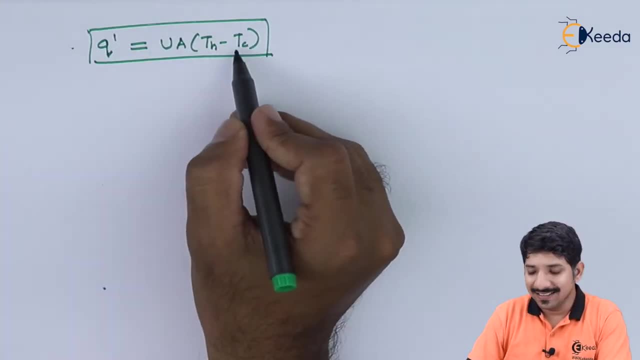 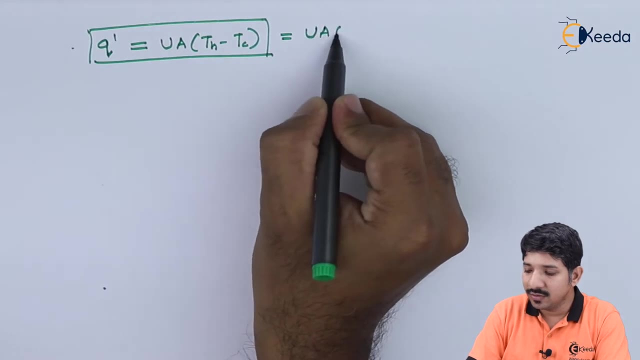 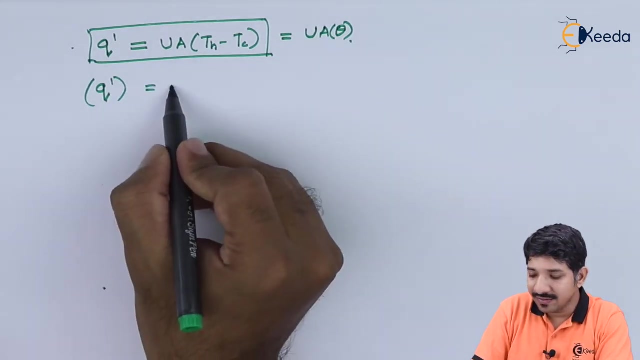 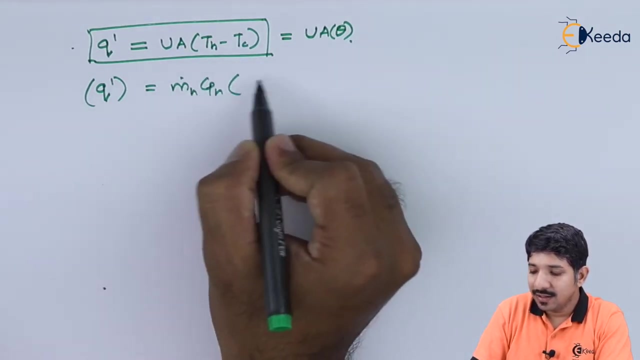 cold temperature is given as TC. So with this we can write this equation and then I can assume that TH minus TC is not nothing but UA into theta. Similarly the value of Q dash also can be given with the enthalpy difference. So that is m dot, H and CPH. 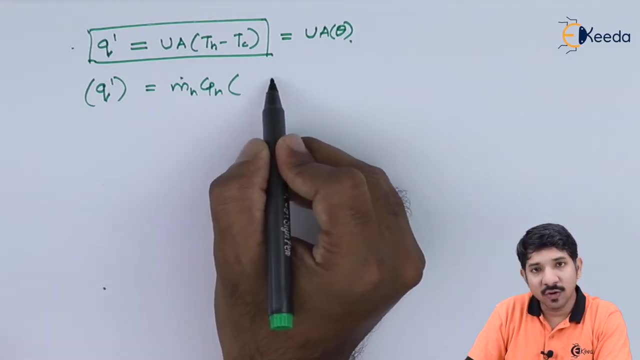 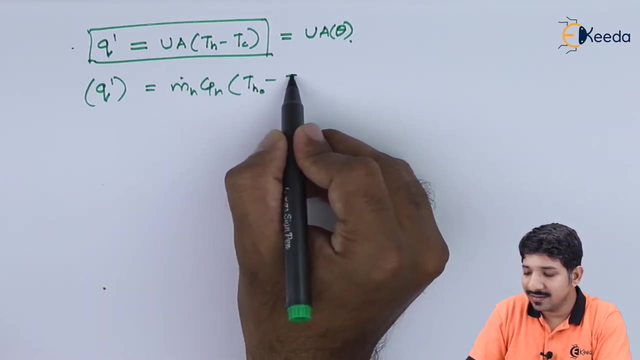 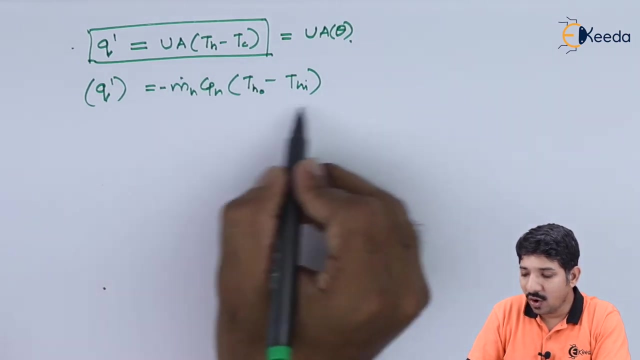 The temperature difference is obviously the higher temperature minus the lower temperature, So that is in this case, the exit temperature is THO minus THI. Okay Now, in this case the heat is lost, So we need to write down the minus sign over here by the hot fluid. 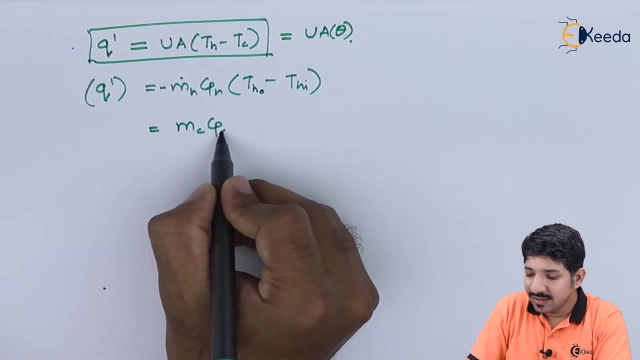 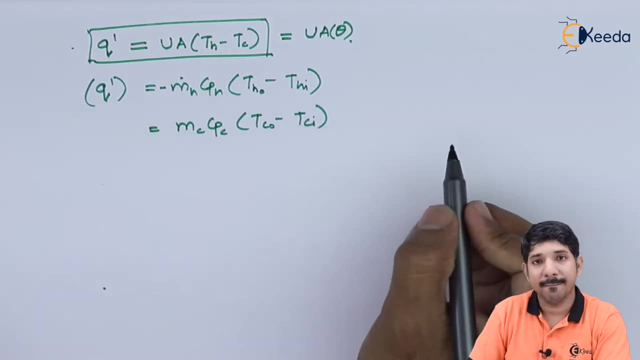 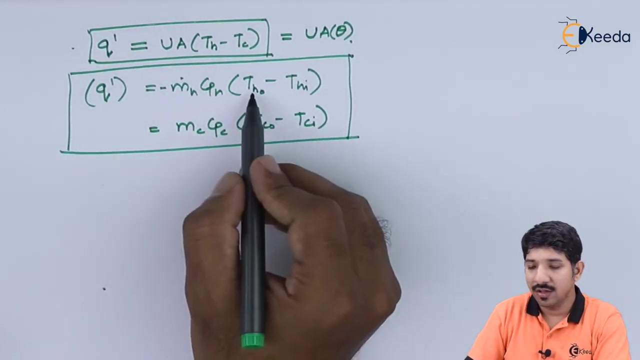 Similarly for the cold fluid, we can write this as MC, CPC. The exit temperature is TCO minus TCI. So this way, basically, we can write down the value of heat transfer rate for the cold fluid and hot fluid and using the overall heat transfer coefficient. 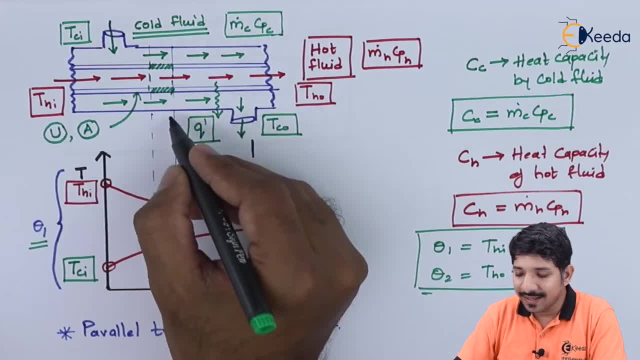 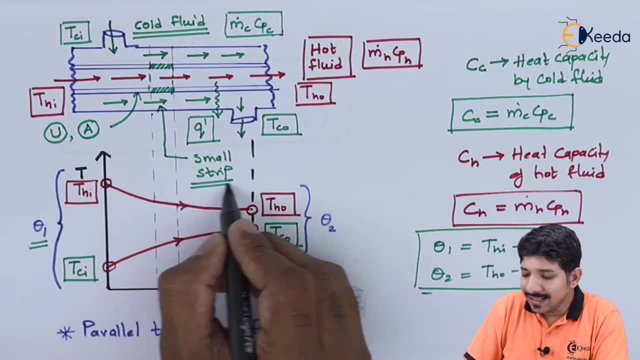 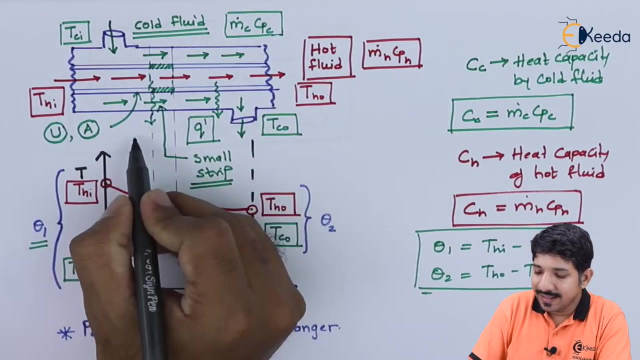 Now, next, what we are going to consider. We are going to consider the heat transfer coefficient. We are going to consider a small elemental strip. So this is a small elemental strip, and then we are going to say that the amount of heat that is transferred is, let us say, dQ dash. 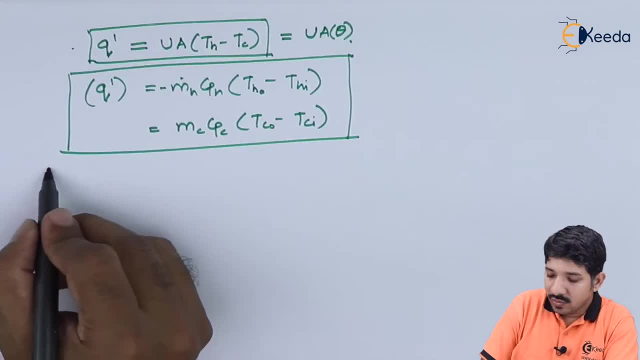 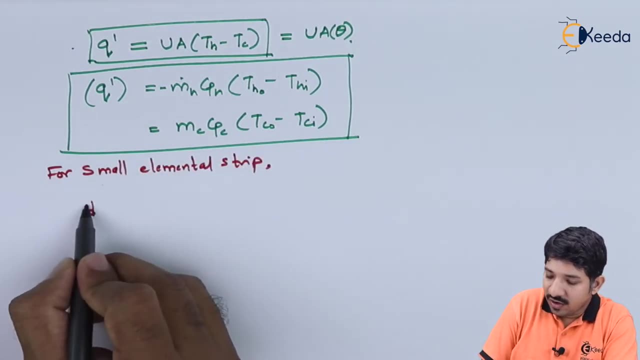 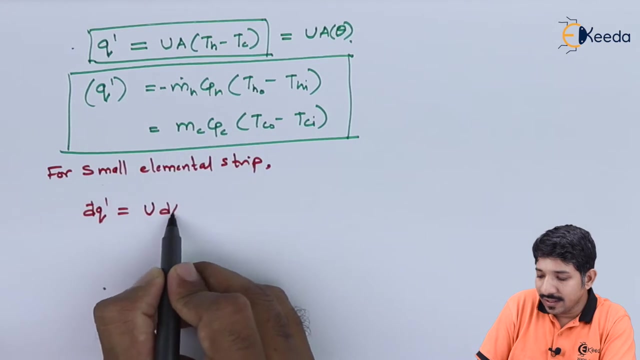 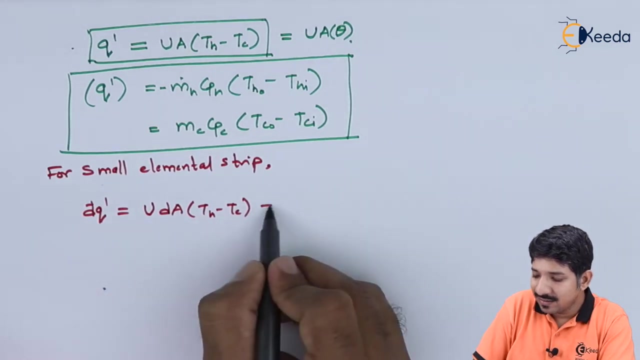 So for this again we are going to write down the expressions. So for small strip The value of dQ is given as again, by this way I can write U into the elemental area can be considered as DA and TH minus TC. So we can write this as U DA into theta. 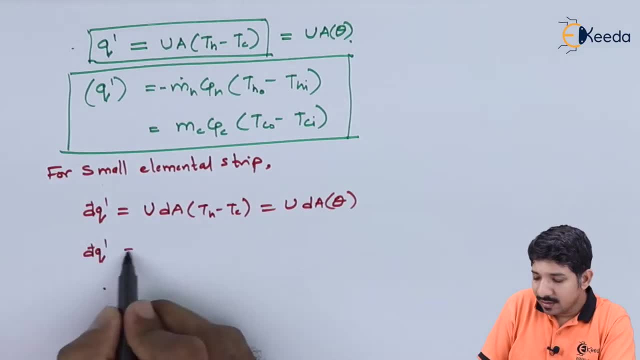 Similarly, we can write this value by the enthalpy difference. Same way. here, instead of this value, we can write down the capacity, So minus THI, Okay. And then we can also write this as U THI minus C H, and here we have the difference. 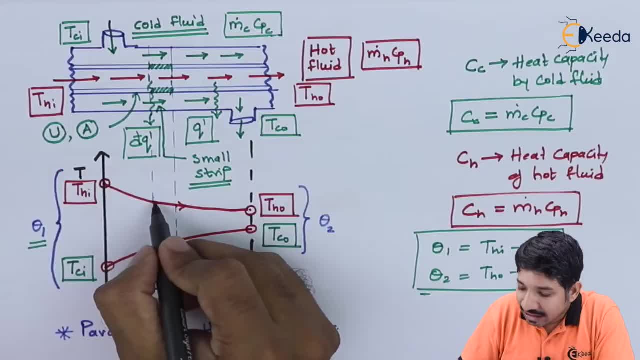 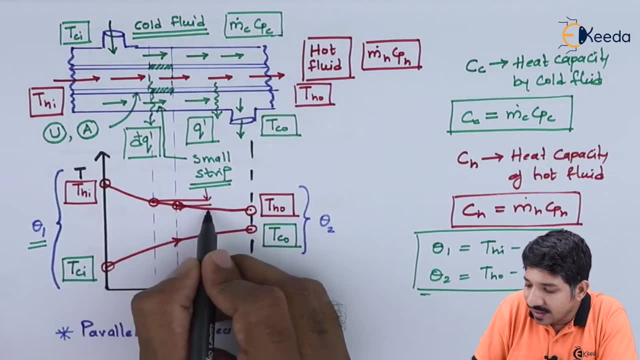 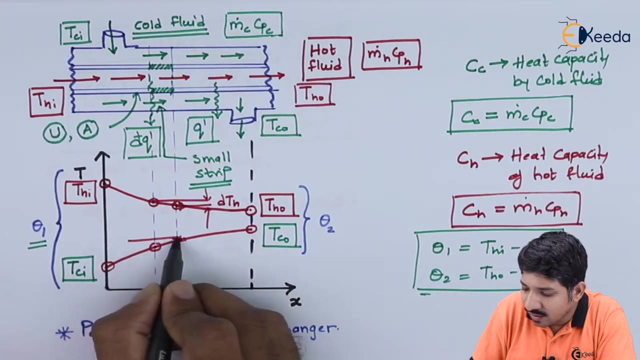 as dt for H. Now this can be seen over here. See, these are the two temperatures. The difference between these two temperature is what we are calling as dth, and the difference between these two temperature is what we are calling as dtc. Okay, 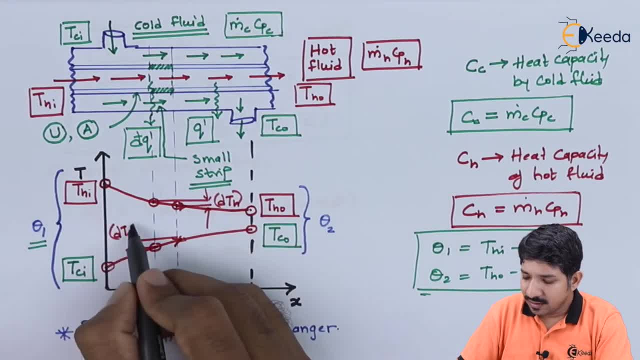 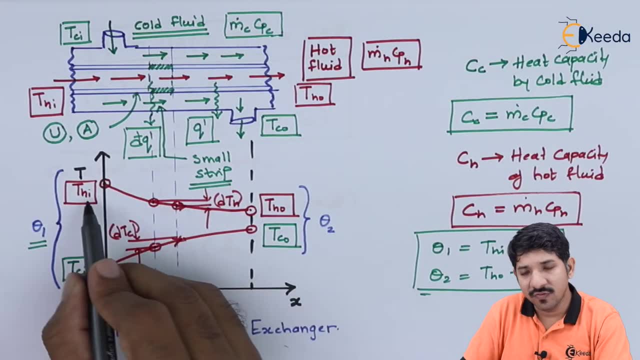 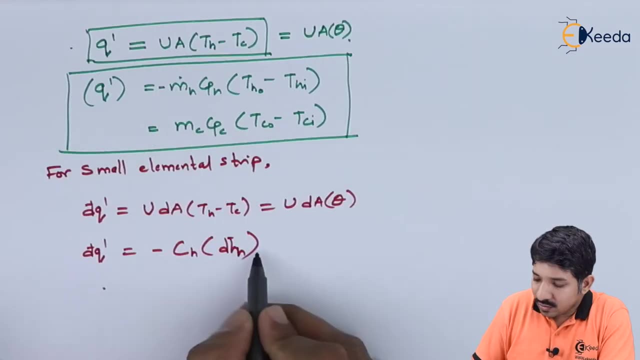 now this is really important to understand that for the elemental strip, obviously there is a, the temperature is decreasing in case of a hot fluid and for the cold fluid the temperature is increasing. now let us write down the expression for the same. so this is for the hot fluid, for the 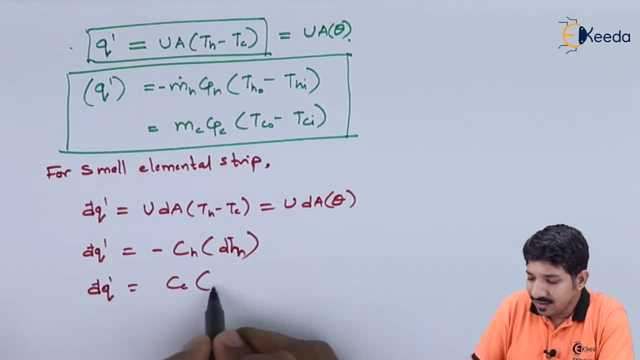 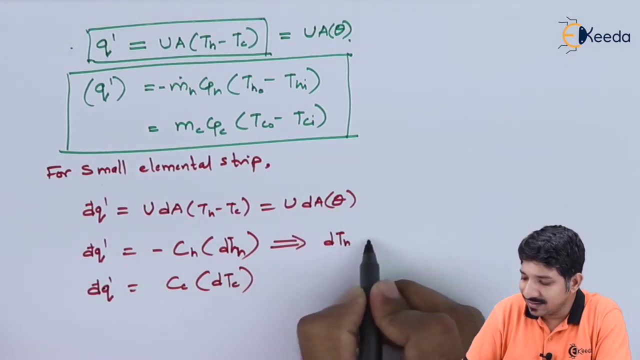 cold fluid. i can write down this as cc, and here we can simply write down as d tc. now again, if i rearrange these two terms, i can write down this as d th, as nothing but dq dash upon ch with the minus sign, and this i can write as d tc, as 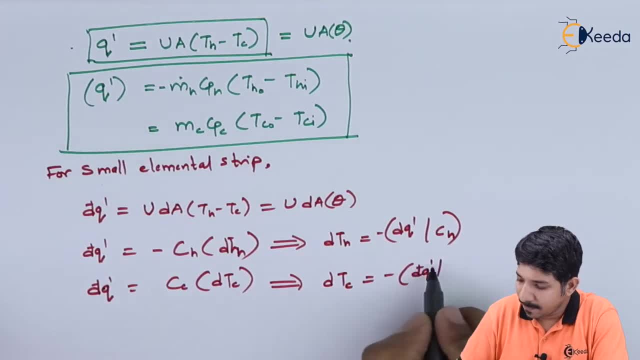 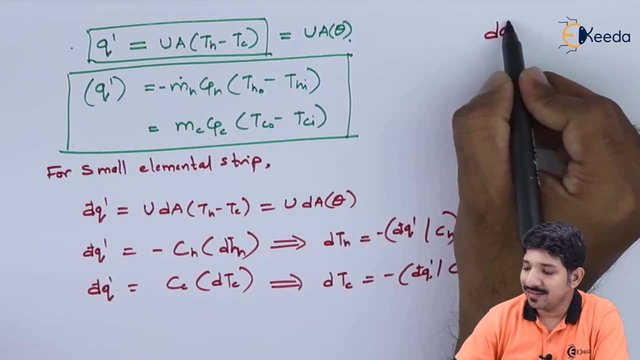 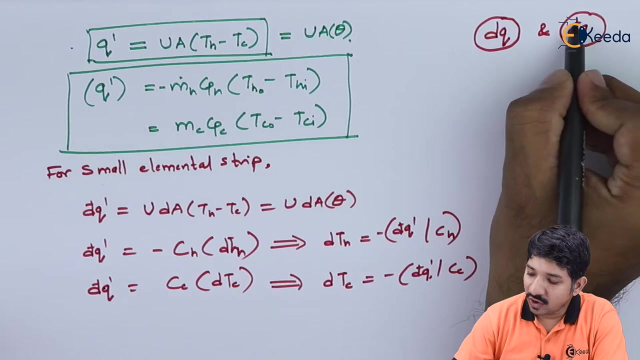 minus sign and this i can write as d tc as minus sign, and this i can write as d tc as minus sign: minus d, Q dash upon C- C. Now try and understand the difference between this term and this term. See, this cross need to be given because this heat transfer rate, that is, this Q dash. 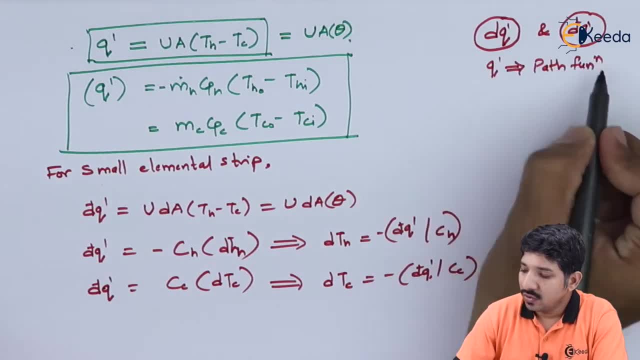 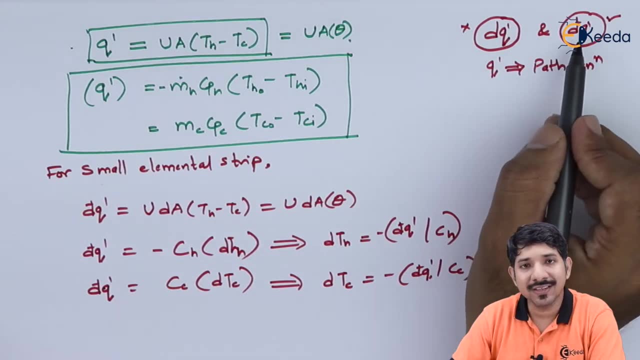 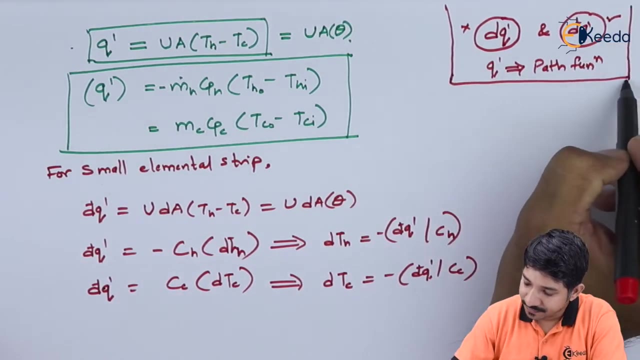 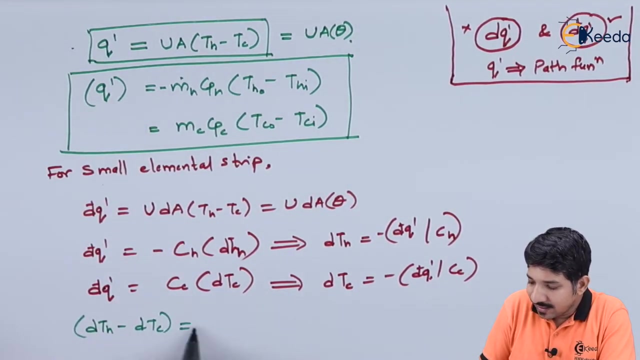 is a path function, So we cannot write this way. This is the only right method of expressing the change in heat transfer rate. Now, this you can understand in the summary itself. Now, if I want to express the value of DTH minus DTC, I can obviously use this expression. 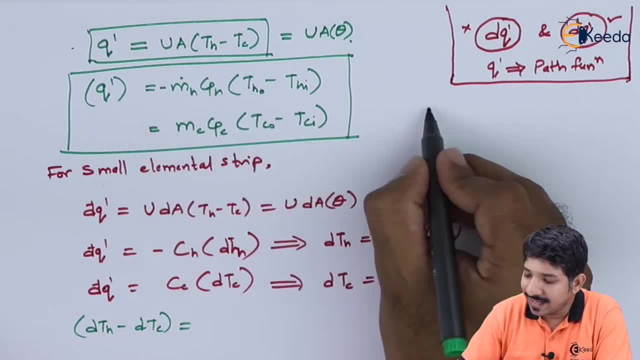 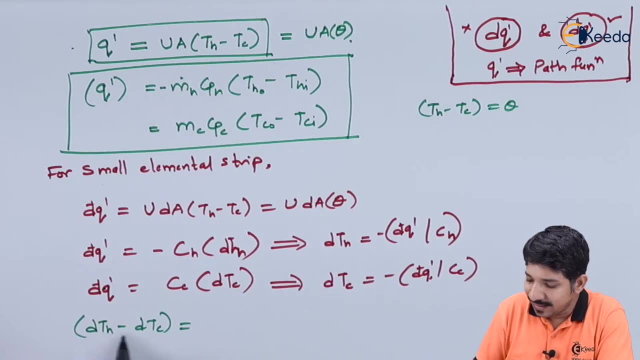 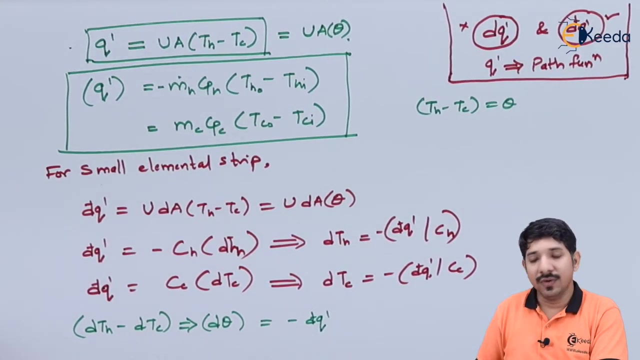 and this DTH minus DTC. as we know that DTH minus Tc is theta, We can simply find out: this DTH minus DTC has nothing but D theta, And then with these equations, I can write down as minus D, dash, Q, dash, and so basically, 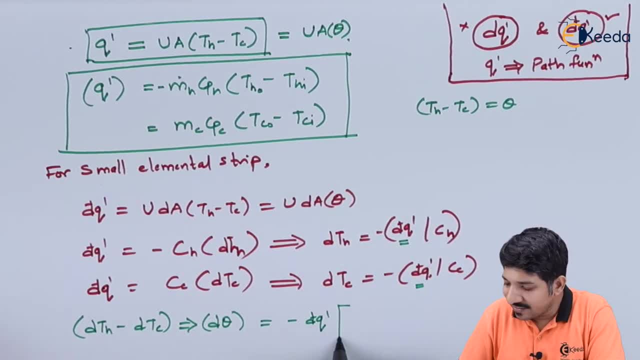 I have taken these two common, So what is left inside is one upon C H, And then the minus sign is over here. This minus sign will get positive, So 1 upon cc. I hope this part is understood. Now. in this case, instead of dq dash, I can write this term: 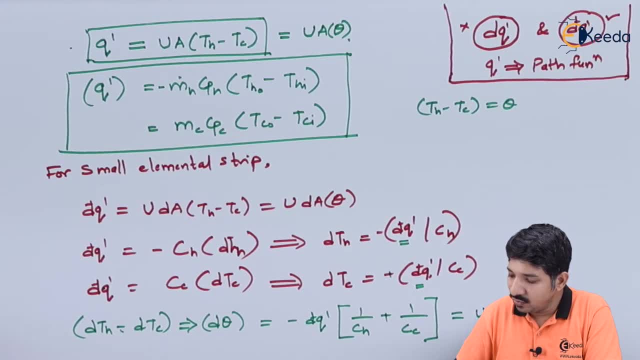 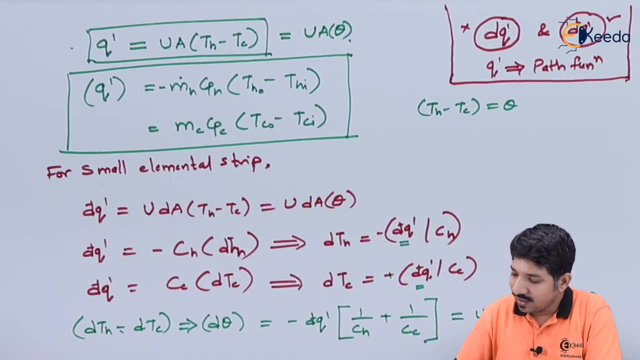 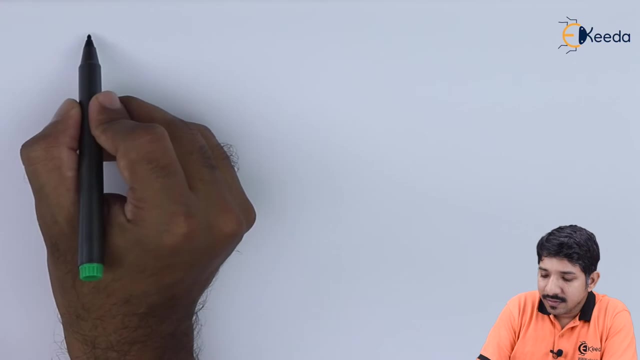 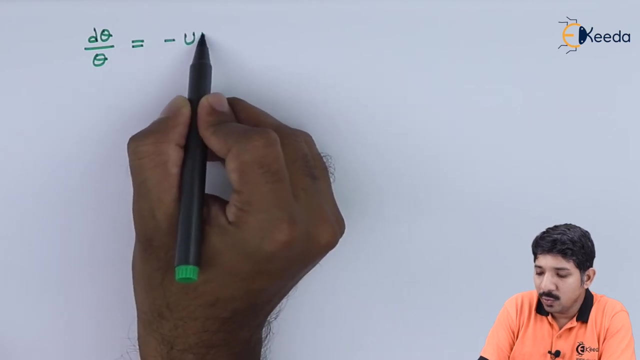 So my final expression will become u into da, into theta, And again the 1 upon ch plus 1 upon cc. Now let us simplify this equation. If I rearrange the term, the previous equation can be written as d: theta upon theta is equal to minus u, a, And we have left with. 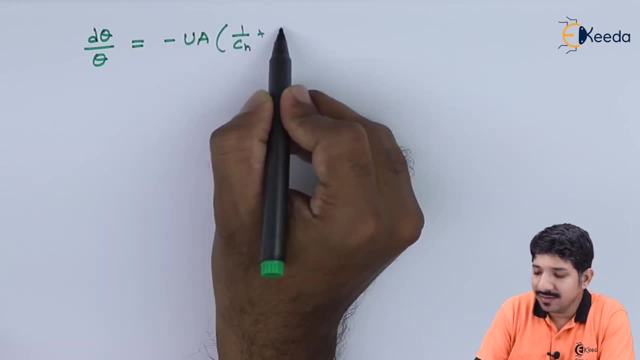 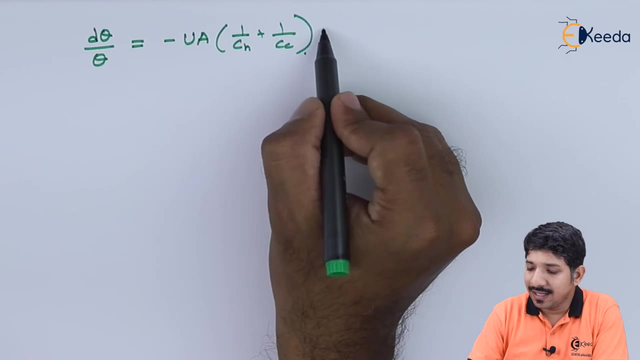 d theta upon theta, And we have left with d theta upon theta And we have left with d theta upon theta, 1 upon ch plus 1 upon cc. Now, in this case, the area will be there with the da term: This area. 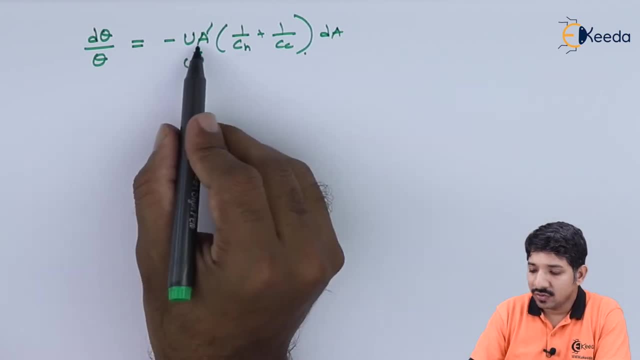 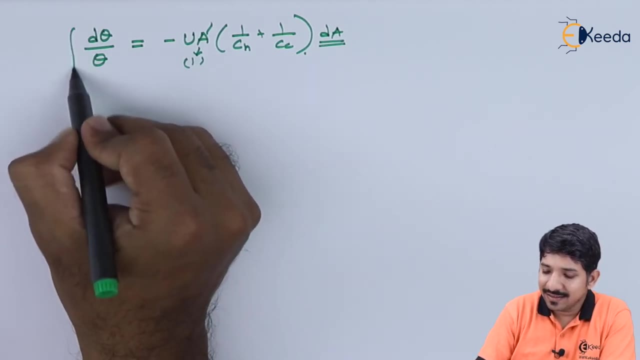 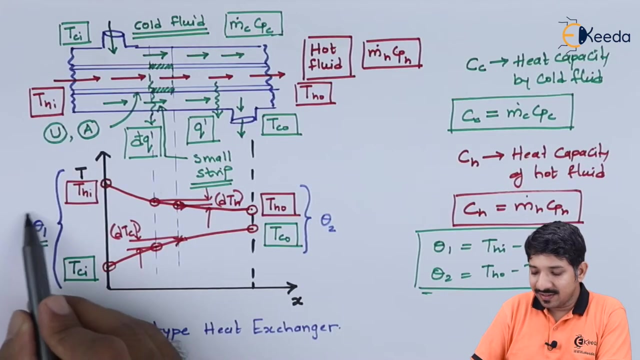 will not be there, So you can consider this as 1.. So, since the elementary area is there, so the da term will come into picture. Now, if I integrate this now, limit for this integration will be: the limit of that integration can be seen from this: 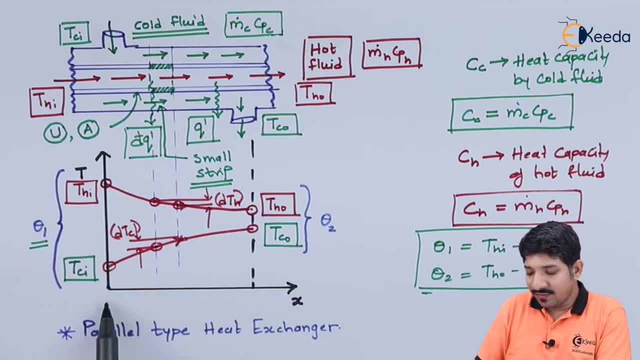 here. So this is the limit of that integration. So this is the limit of that integration, The value of area increasing from 0 to a- over here, Okay- And the value of theta is increasing from theta 1 to theta 2.. So if I put those limit, I can write this as theta 1.. This is theta 2.. This. 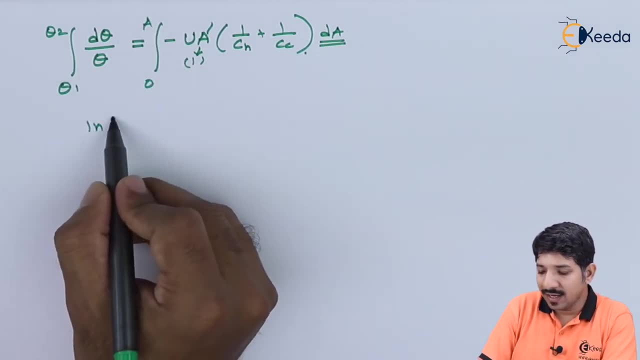 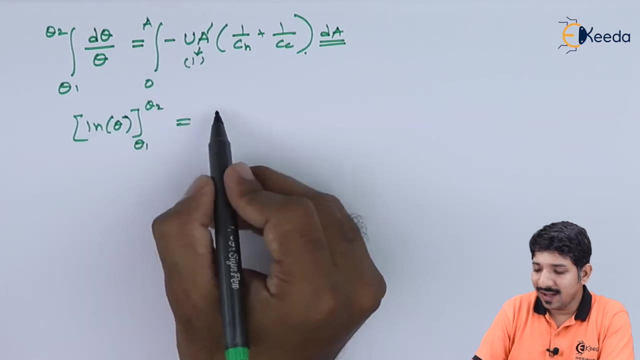 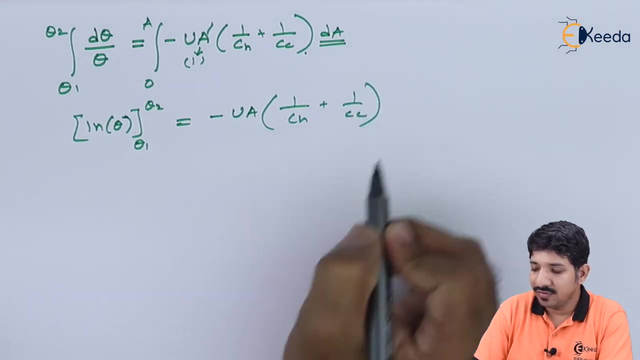 is 0.. This is a, So my simplification will be ln of theta, with the limit theta 1 to theta 2.. And here I will be left with minus u, a And, in the same term, 1 upon ch plus 1 upon cc. So again I can write this as ln of. 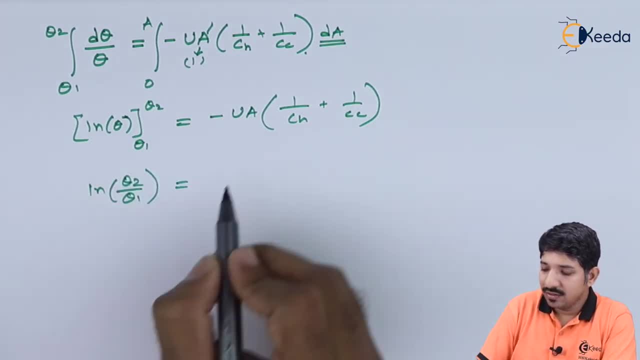 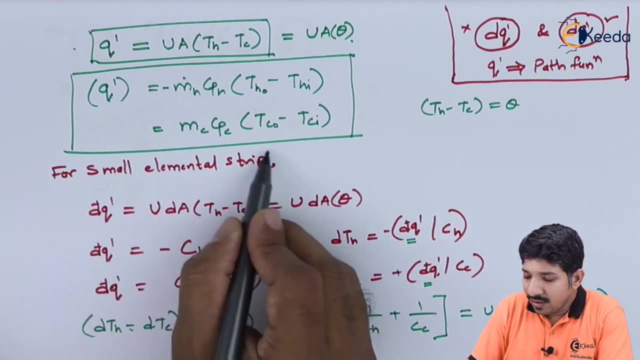 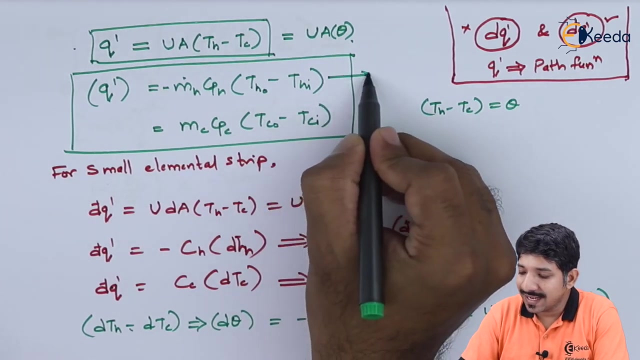 theta 2 upon theta 1, which is equal to minus u a. Now let us try and simplify this part. See, before we have written for the small elemental stream, for the whole heat exchanger, we can write this expression as minus ch. 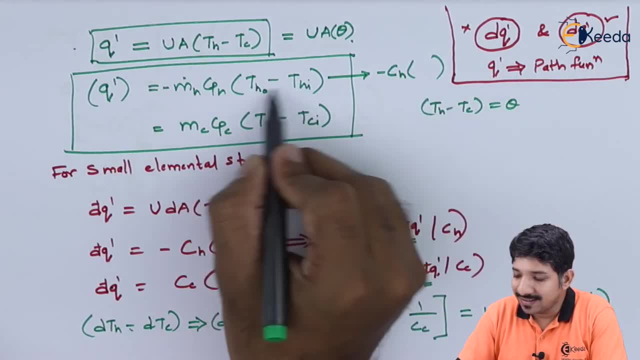 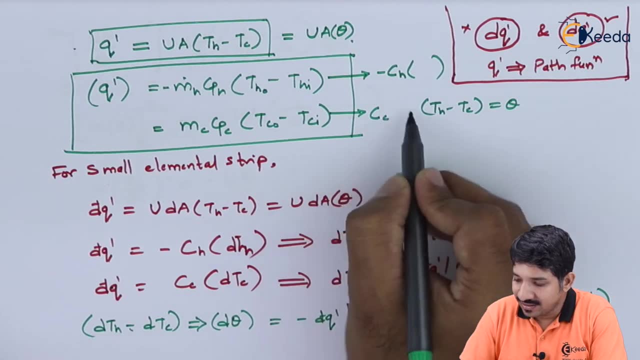 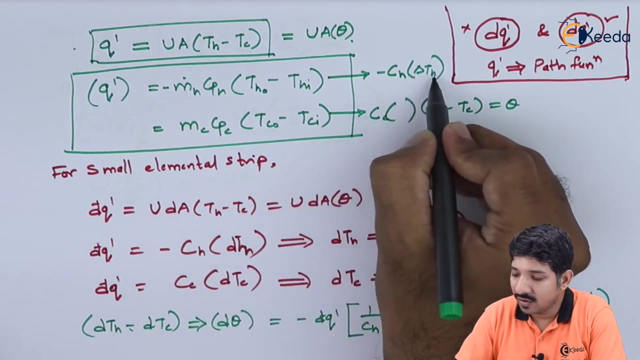 In the bracket, again this delta t, And here also we can write plus cc, And again the same, the delta t value for the cold fluid. So let me write the delta t for the hot, the delta t for the cold fluid. Now, with this we can write down the value of ch as q dash upon. 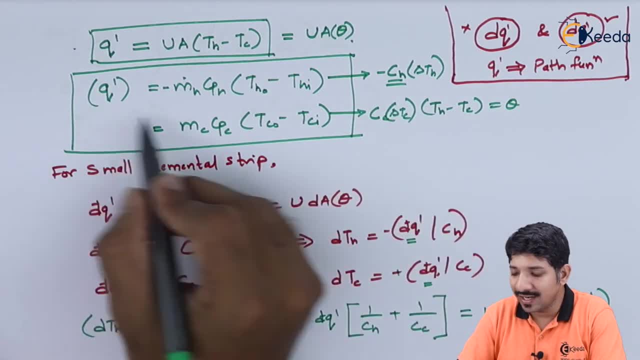 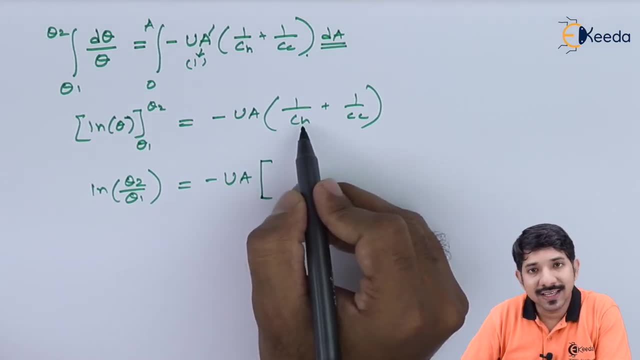 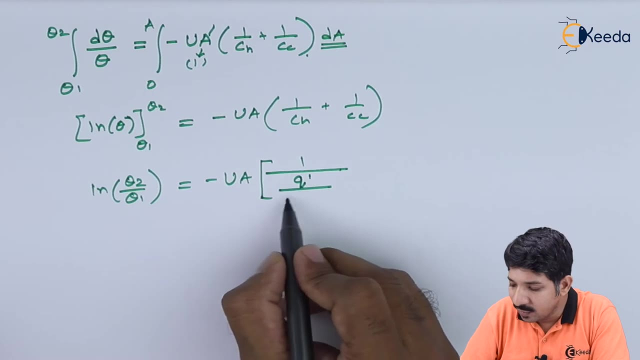 the delta t for the hot and the value of cc as q dash upon the delta t for the cold fluid. So if I do so, I can write the value of ch as 1 upon q dash upon the delta t for the hot fluid. 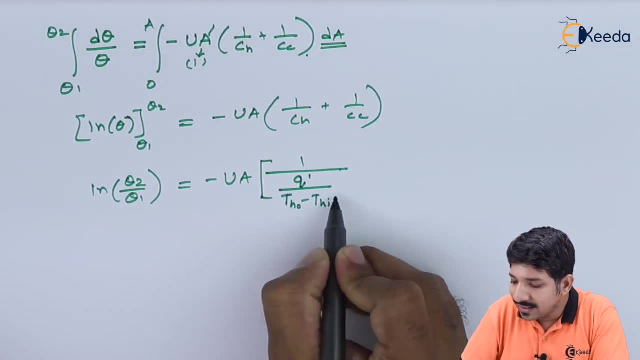 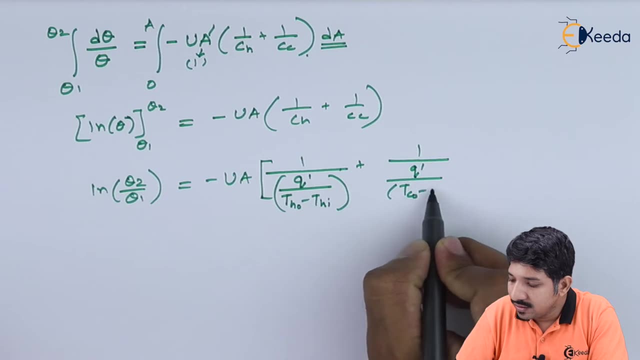 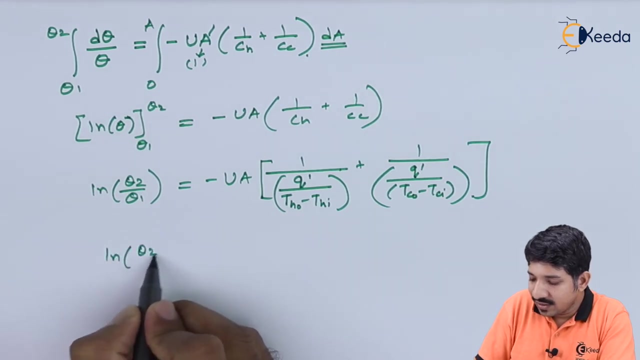 So this we have written as th o minus th i plus 1 upon q dash upon tc o minus tc o. So again, if I rearrange those terms I can write this as ln of theta 2, upon theta 1 is equal to minus u a. this q dash can be taken outside and it can be written at: 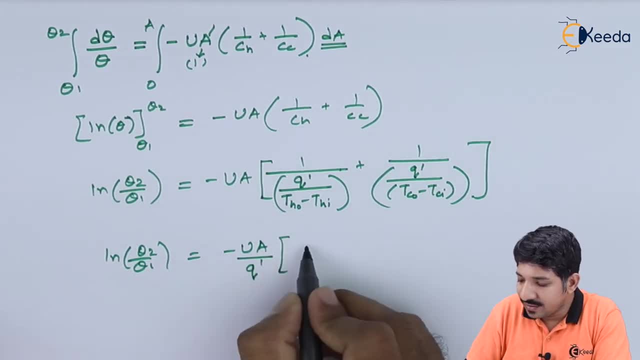 the denominator q dash. So what do we have here? THI minus THI plus TCO minus TCR. Now, if I rearrange this term, I can write down this equation itself. as q dash is equal to now, this minus sign can be taken inside and we can rearrange the entire term to write down this. 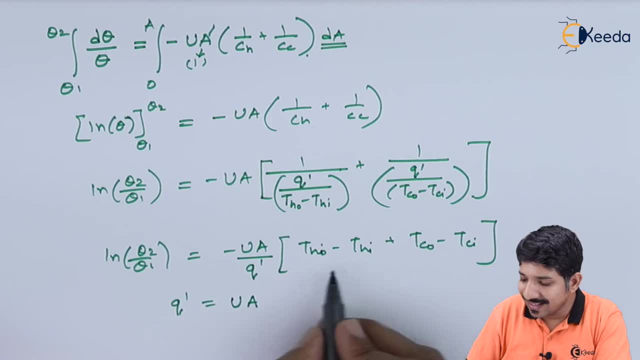 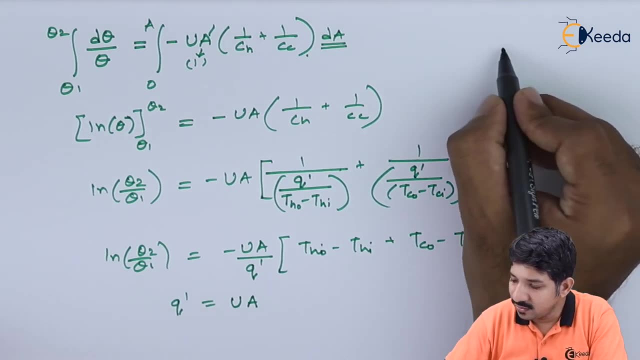 as u into a and if I take this minus sign inside, what do I have? I can write this term as nothing but theta 2 minus theta 1.. What is theta 2?? From this expression, theta 2 is nothing but THO minus. 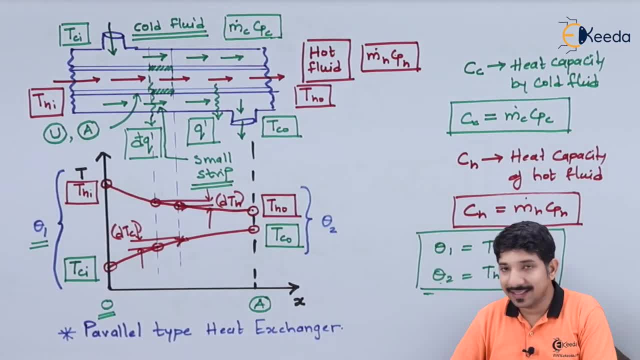 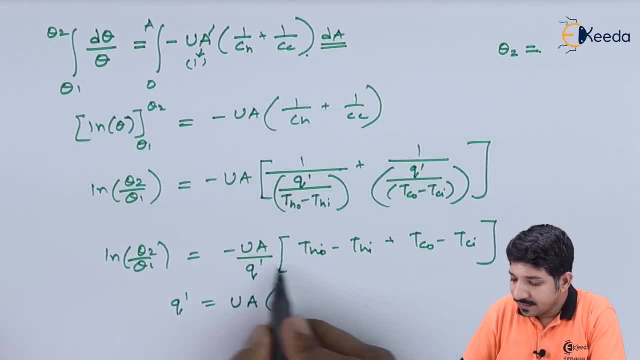 TCO and theta 1 is nothing but THI minus TCI. So what I can do is I can rearrange those term, see here minus sign. if I take it inside, I can write this as minus THO plus THI, minus TCO plus TCR, and obviously in the denominator ln of theta 2 upon theta 1.. 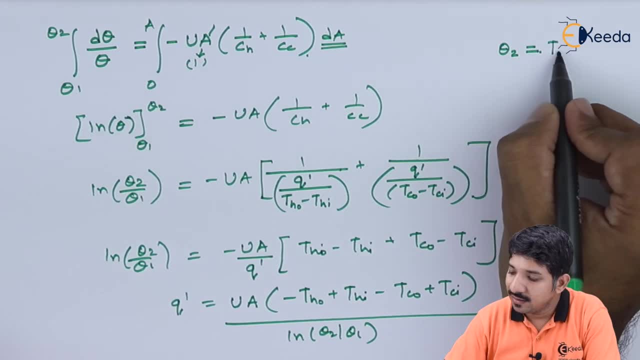 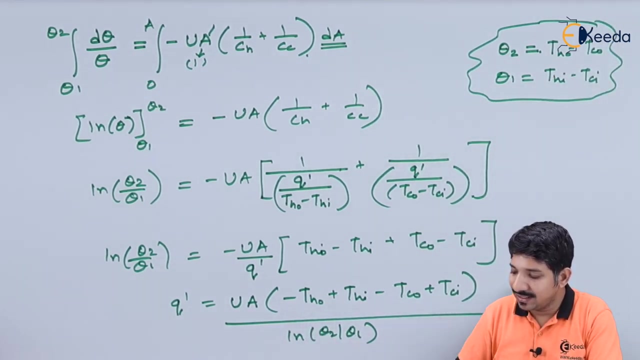 Now theta 2 is written as THO minus TCO, theta 1.. Now theta 2 is written as THI minus TCI. So if I use this, then with the help of rearrangement I can write this as nothing but theta 2 minus theta 1.. So finally, I can write the equation. 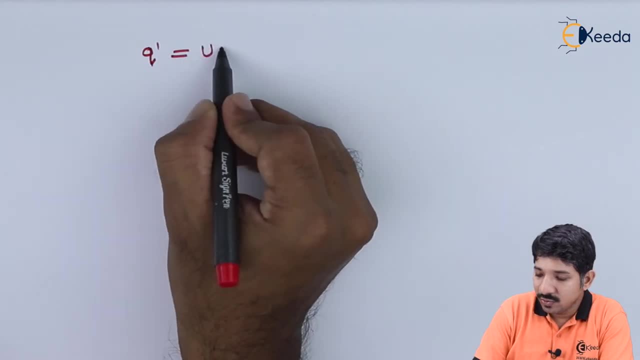 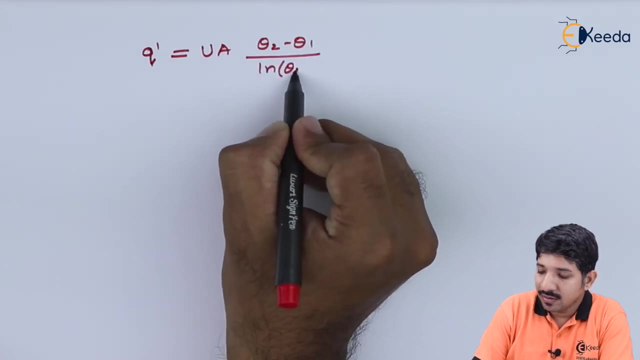 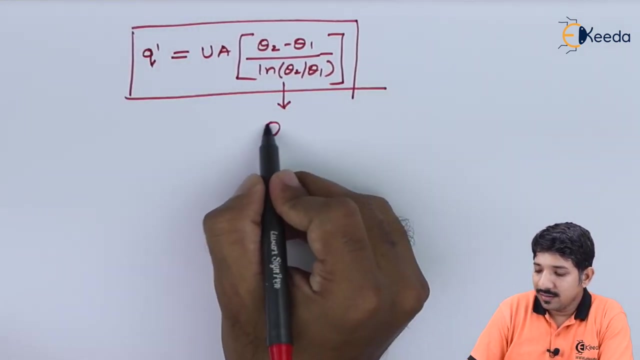 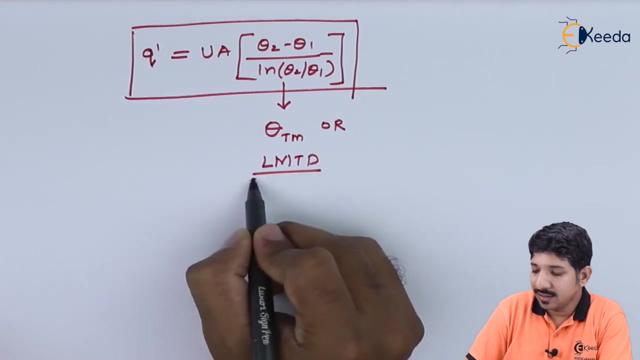 as the heat transfer rate is given as u a theta 2 minus theta 1 upon ln of theta 2 upon theta 1. call as theta TM or LMTD. So that is log mean temperature difference. So if I know for a